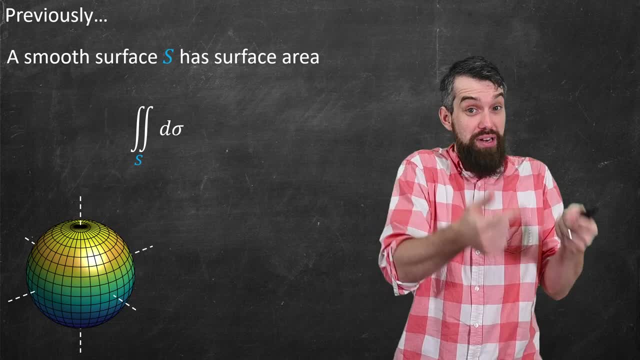 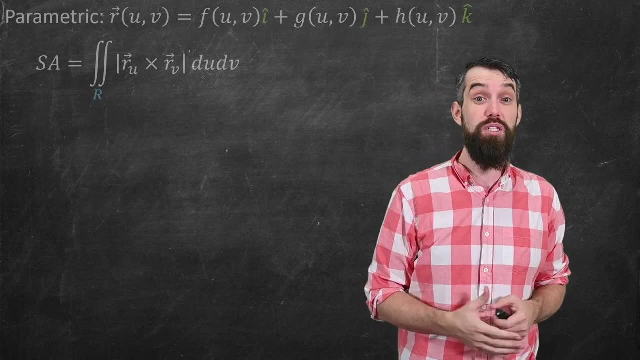 arc length parameter ds, which was great for definitions but wasn't how we typically computed things. So in our previous video we've talked about how to compute this in a few different cases. First, there was parametric. If your surface was described parametrically, some position. 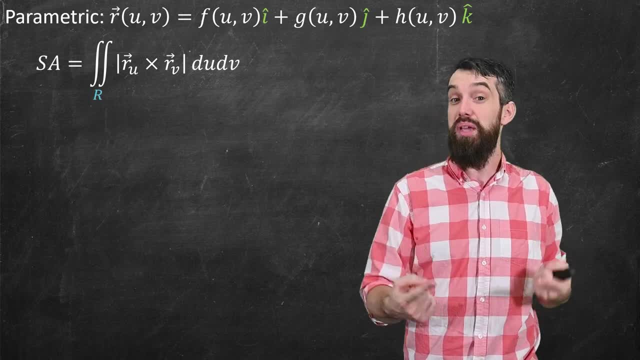 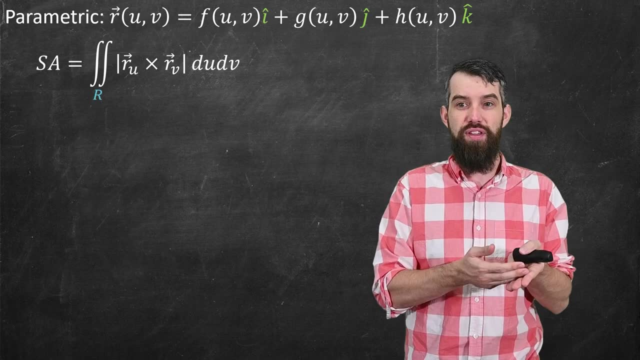 function r in terms of u and v, then your surface area could be computed by taking the double interval of your integrand being the length of the cross product, our u cross, And so the combination of the cross product and the du dv is our little element of surface area. 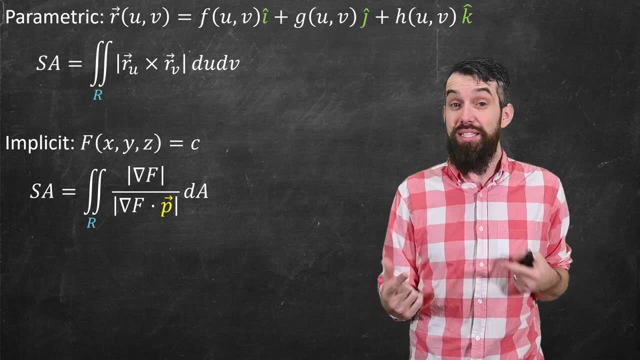 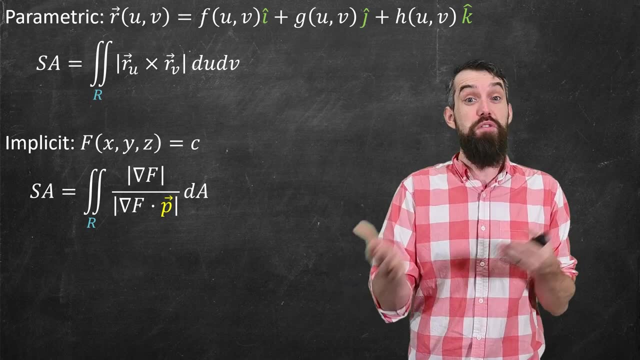 when it's described parametrically. Alternatively, it might be described implicitly with some big function capital f of xyz equal to c, a level surface, And when that was the case, we've previously seen the surface area could be written as the double interval of the length of the. 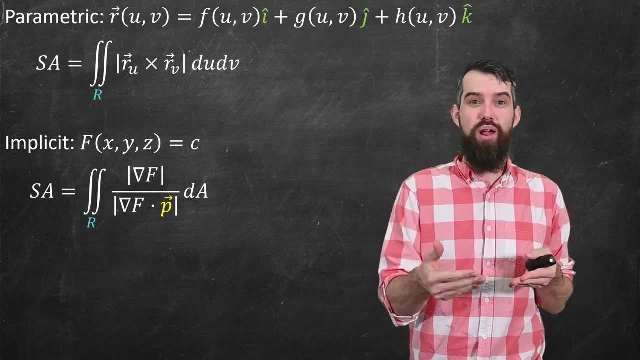 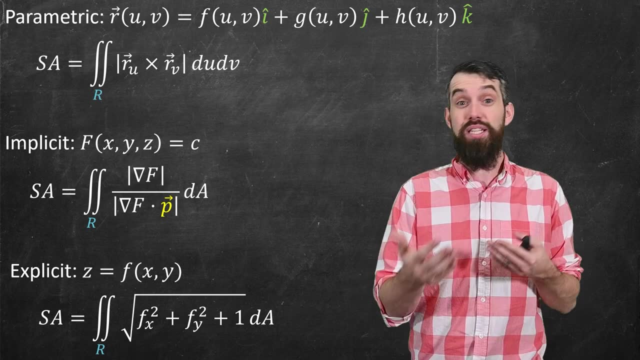 gradient of f divided by the absolute value of the gradient of f, dotted with the vector p, which was often k? hat but could be i hat or j hat as well. And then, finally, we saw that when it was described explicitly, z, as a function of xy, it could be: 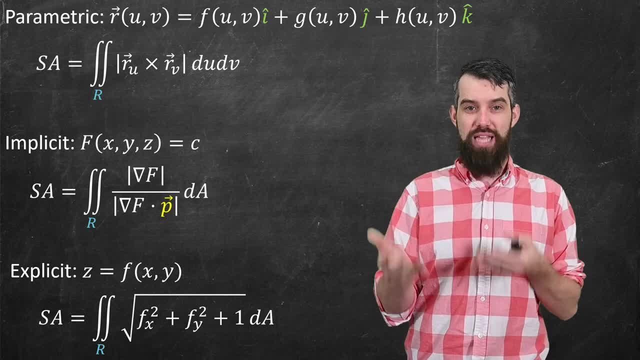 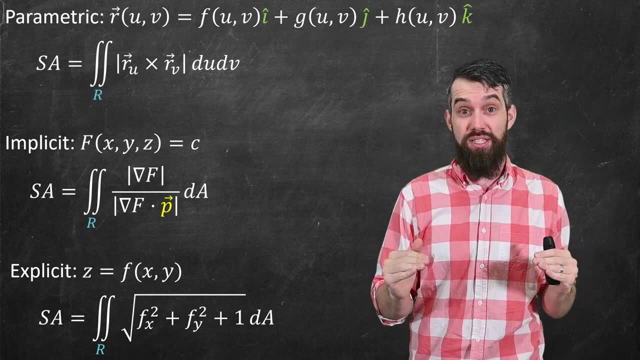 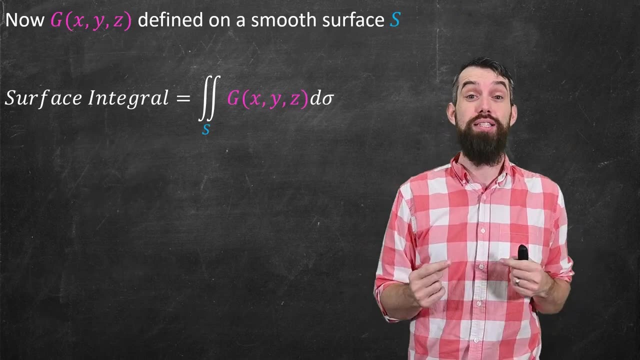 described as double interval of square root, of fx squared plus fy squared plus 1.. So the point is: three different ways to describe a surface, three different methods to compute out the surface area of that surface. Okay, so that's what we did in the past. Now let's go to the concept of a surface integral. 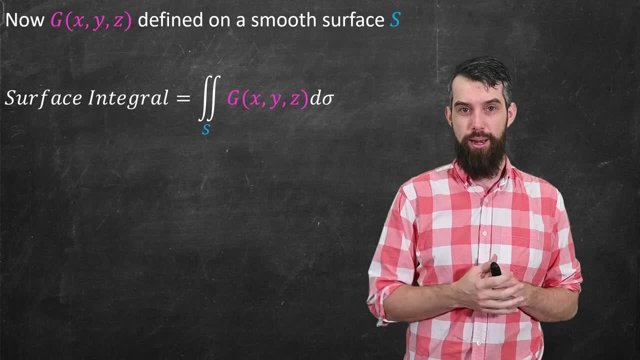 And the idea here is: I have some new function- I'll call it capital g- of x, y and z, And this is the function that is a function of x, y and z, And this is the function that is a function of x, y and z, And this is the function that is a function of x, y and z. 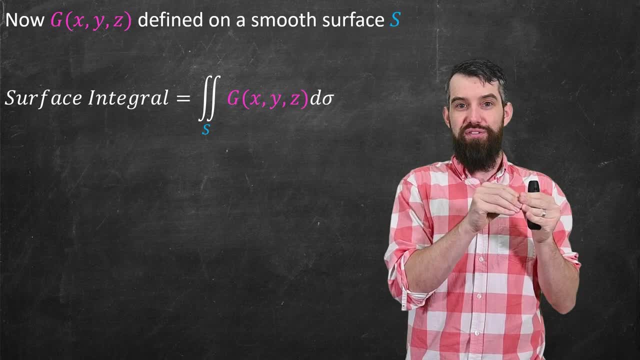 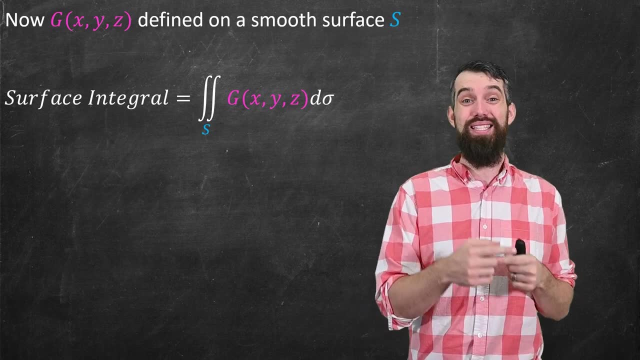 And this is the function that is defined on that surface. So at any point on the surface there is a height, if you will, the value of this function, g of x, y and z. It's a little harder to visualize this as a height now because your surface might live in three dimensions. 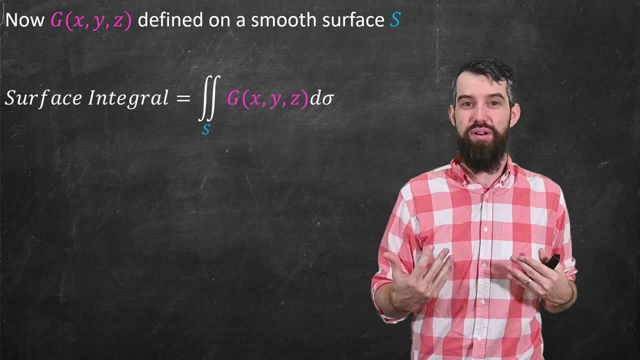 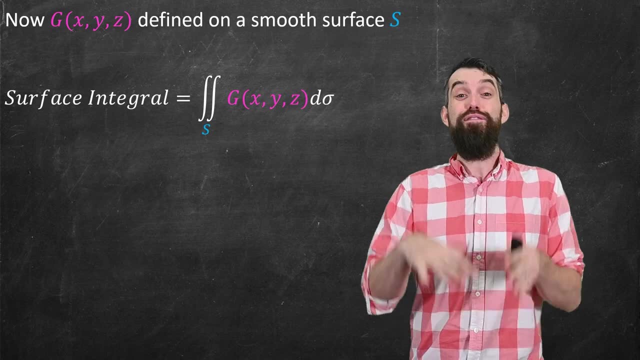 so the graph of this would be a four-dimensional object. But regardless, I want you to think: at any point along the surface there's some value of the function. Then a surface integral is adding up the values of that function along each little element of surface area. That 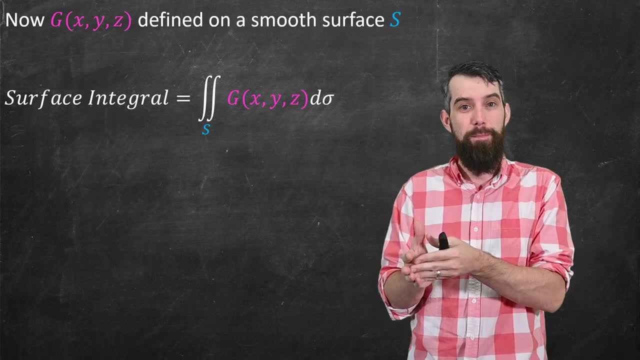 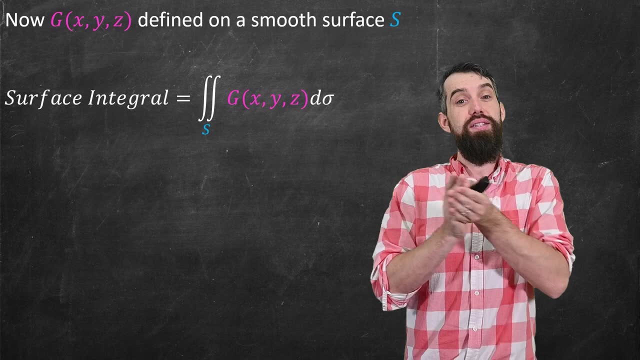 is a double integral along the surface of the function g d sigma. This is exactly analogous to the concept of a line integral, which would be the integral of some function ds. And then I can return to my three different ways of describing it. And two things have changed. 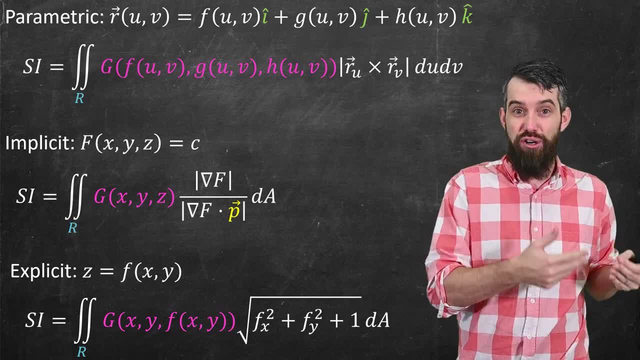 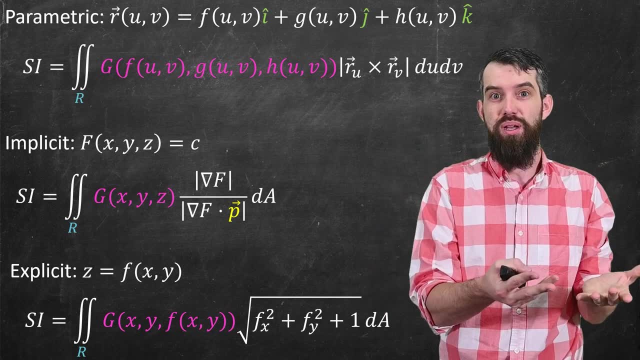 First, instead of surface area, I'm writing si for surface integral everywhere. And then I've gone and I've put a g into the integral in every spot, So this is double integral of g times, whatever the d sigma is for the three-dimensional integral. And then I've 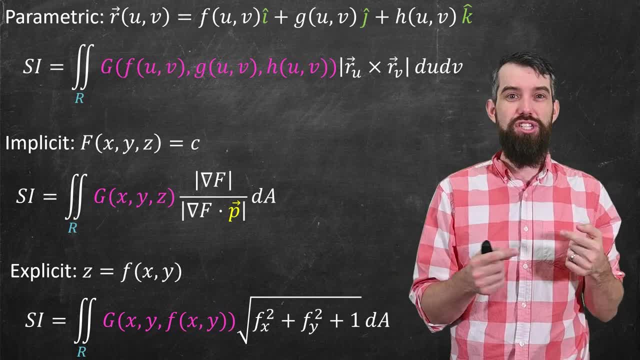 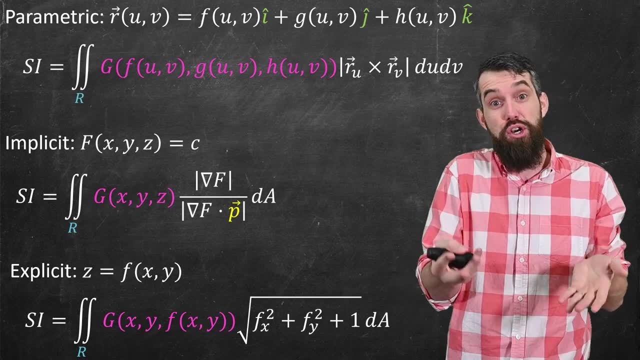 got the three different presentations. The g's look a little bit different and it's just to reflect the type of computation I'm doing. So when it's done parametrically, the three different components are written in terms of the parameters f of u and v, g of 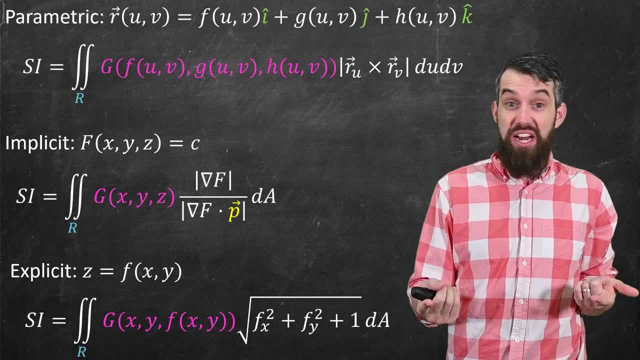 u and v and h of u and v. When it's implicit, you can just write it in terms of g of x, y and z, as we had before. That's fine, And when it's explicit, well, since the z is f. 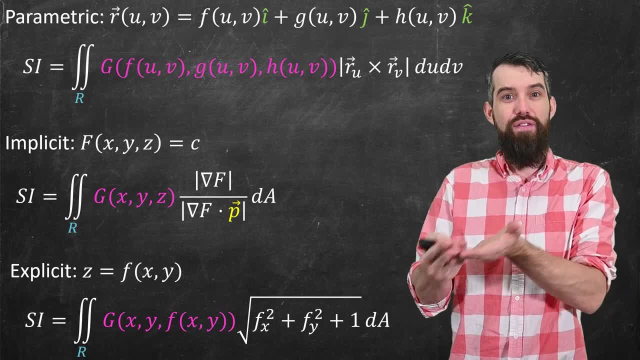 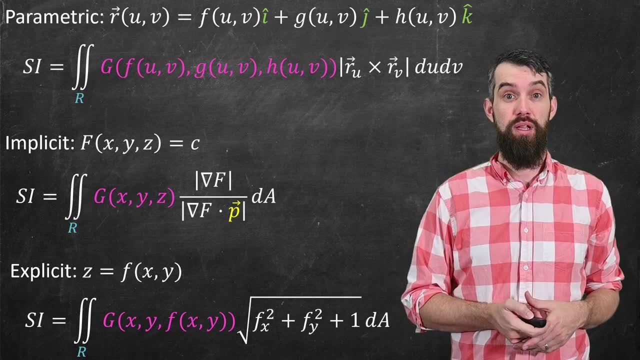 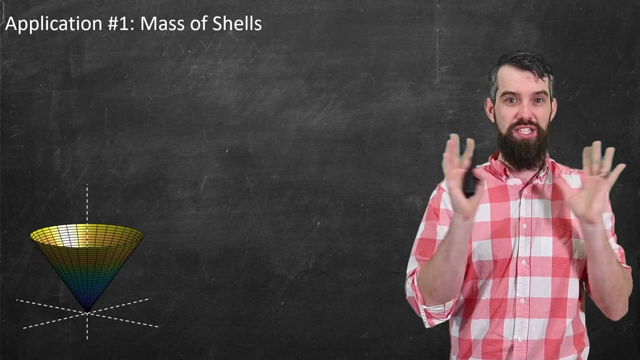 of x- y, I'll write g as x- y and f of x- y in for the third component. Regardless, it's just putting a g in to each of these different places. Okay, so let's see a couple applications. First application is the mass of some surface. 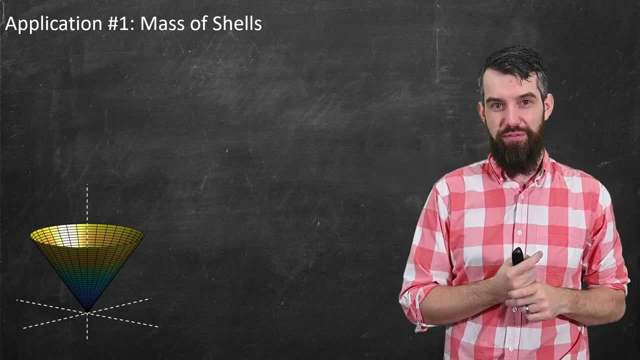 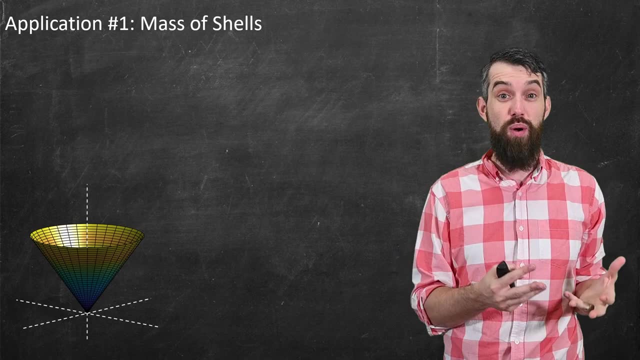 some thin shell, For example. I've drawn this cone surface And I want you to imagine that at some spots this material that's used to make that shell is thicker than at other spots. For example, if you're making a pottery bowl that's spinning on a wheel, some points you 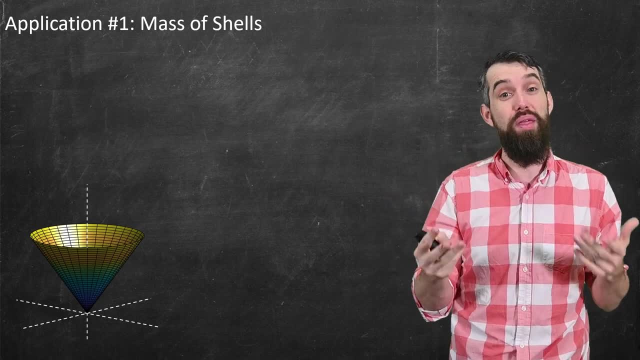 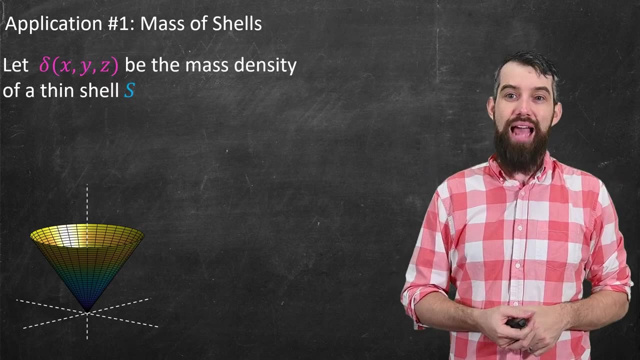 squeeze in and the wall is thinner. Some spots it's a little bit thicker, So you can have a sort of a variable density, a variable thickness as you go along. So then, if you had that, so I'll let delta of x, y and z be the mass density of my thin shell. Then 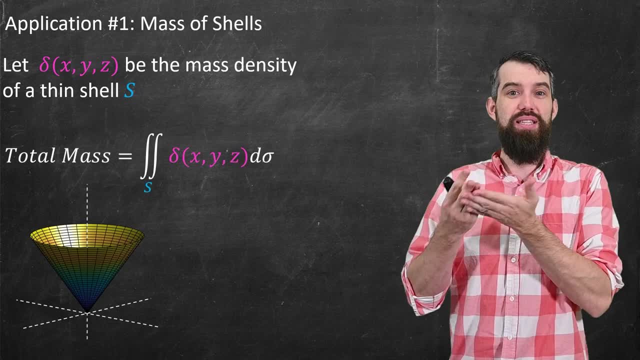 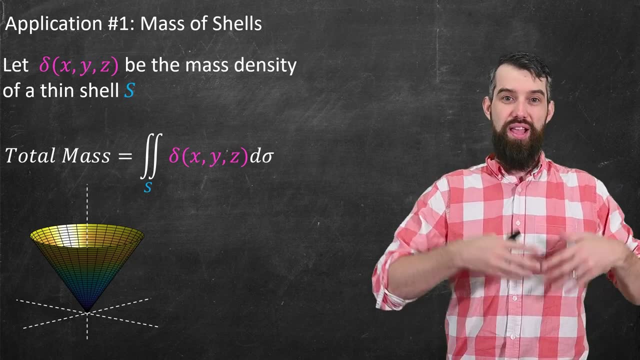 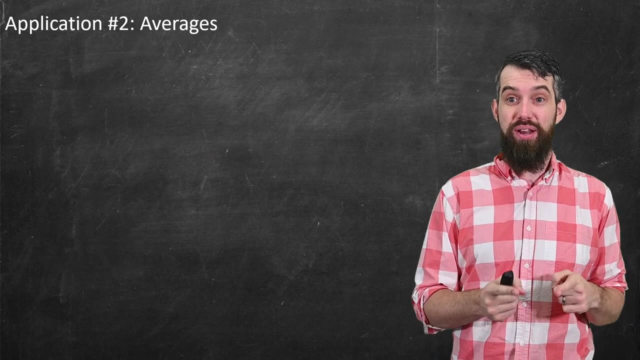 the total mass would be adding up the density times the area, So in other words it would be a surface integral, That is, the double integral over the surface of integrating this density function, the sigma that is for a little element of surface area. A second example: 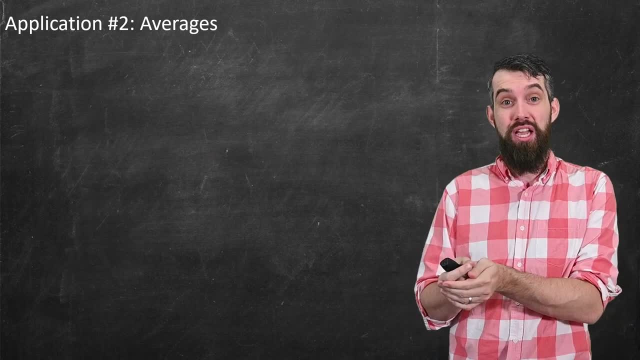 I'm going to use is this The surface area of the cone surface. So I'm going to use a is actually involving a type of averaging, So I want to imagine that there's a temperature at any point on the surface of the Earth. 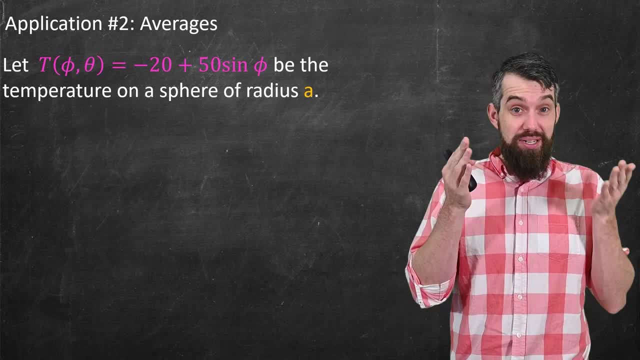 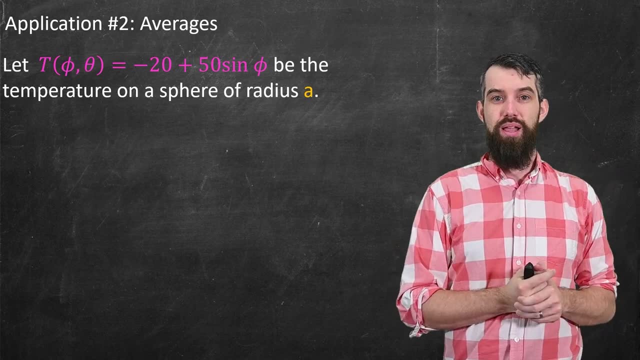 Imagine that's a sphere of radius A, I'm going to assign a particular temperature. It's kind of like saying: you have a height above the Earth, except instead of height it's a temperature above every point on the Earth. And then I just made up some sort of 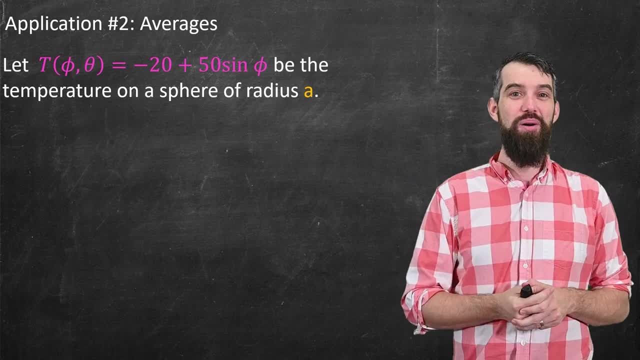 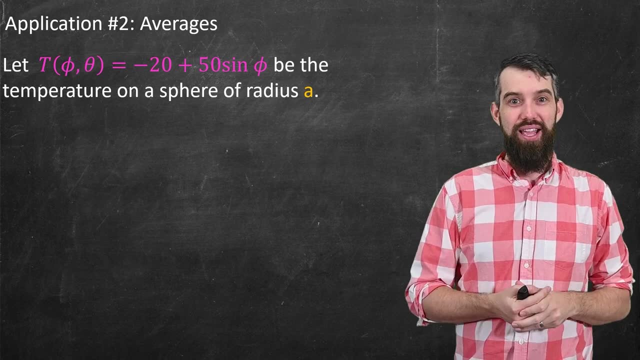 quasi-realistic temperature function. It's really not that good. But I'm basically just saying that if phi was zero or pi, so the North and South Pole- the temperature would be minus 20.. If phi was pi, over two AKA along the equator. 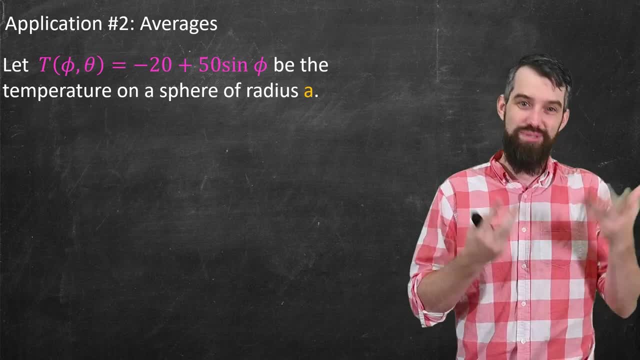 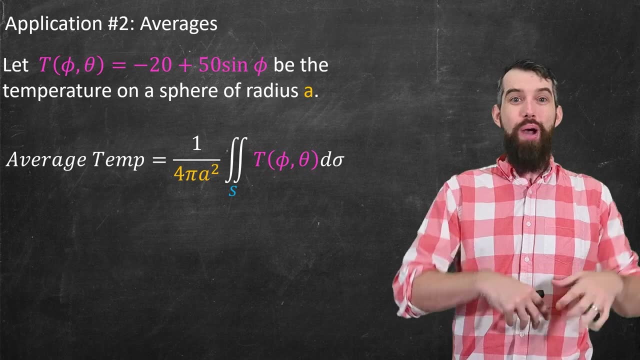 then the temperature would be minus 20 plus 50,, which is 30.. Okay, sort of worked, I guess. Anyways, if I want to figure out the average temperature, well, what's the formula for any average? It's you add everything up. 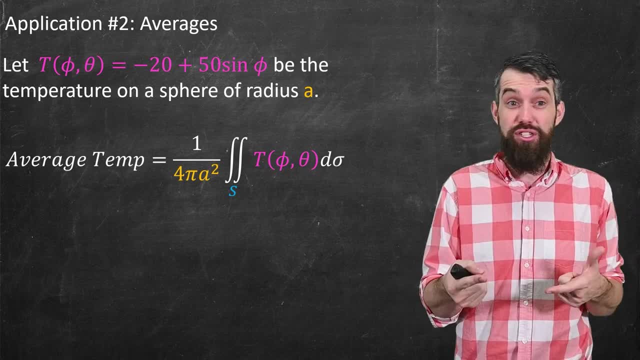 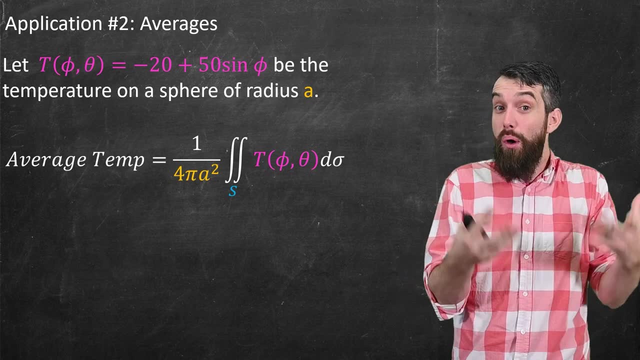 and then you divide out by the number right. If I wanted to compute the average grade in the course, I'd add up all the scores, divide out by the number of students. So the average temperature here is. I'm going to add up all of the temperatures. 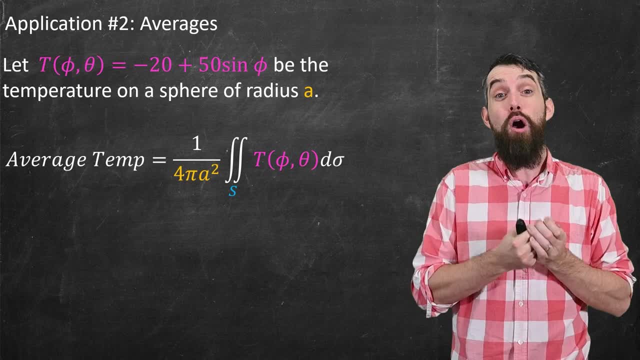 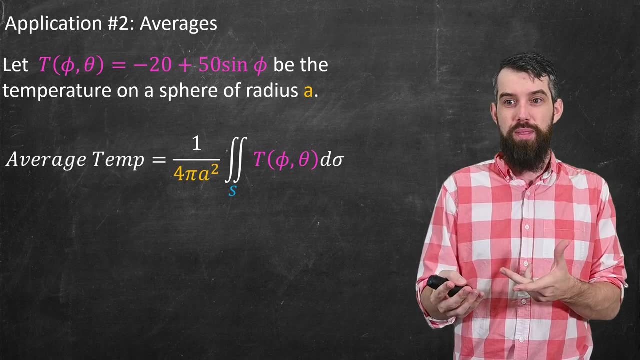 on all of the little elements of surface area and then divide out by the total surface area. So the one over four pi a squared is me dividing out by the total surface area, And then I've got this surface integral where I'm adding up all the temperatures. 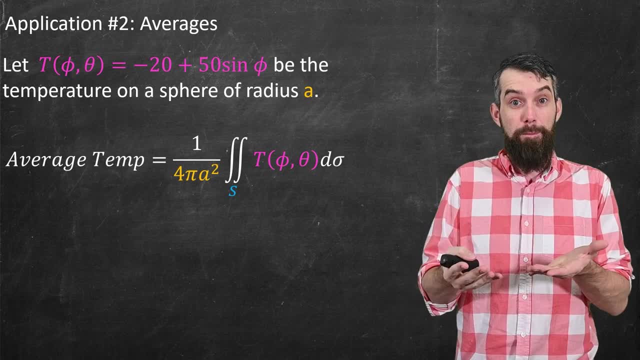 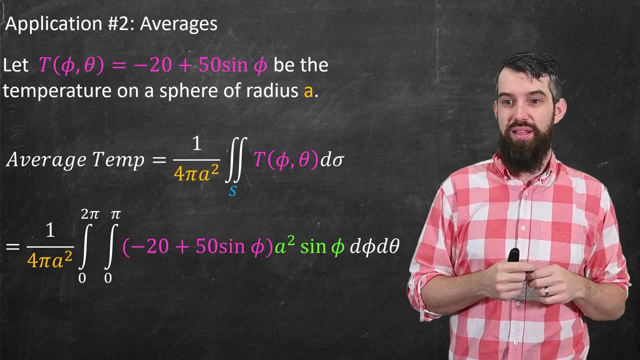 the integral of the temperature function d sigma. Okay, so now I want to compute that out, So I guess I should put in the actual temperature function I have. And then this is described parametrically And imagining my surface here in the phi theta parameters. 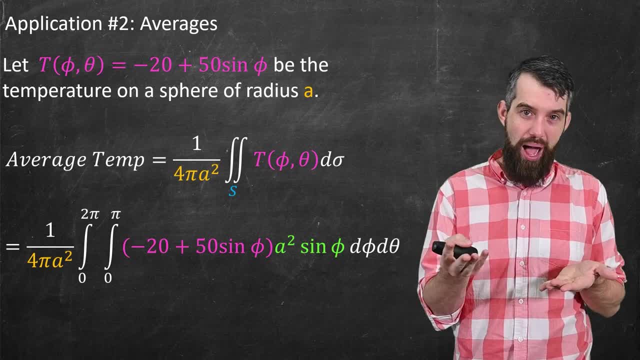 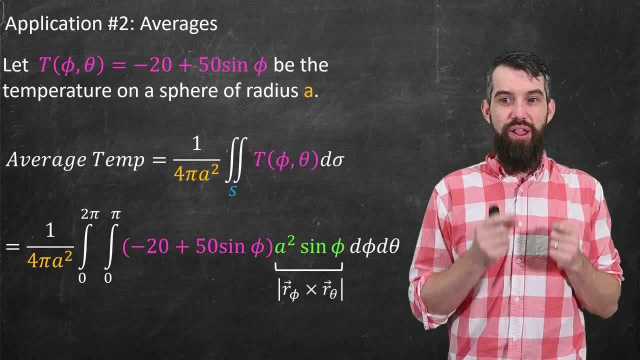 And so I know what they are in spherical coordinates: the phi going between zero and pi and the theta between zero and two pi. And then, the most important part here that's being added, is this: a squared sine phi That corresponds to r phi cross, r theta. 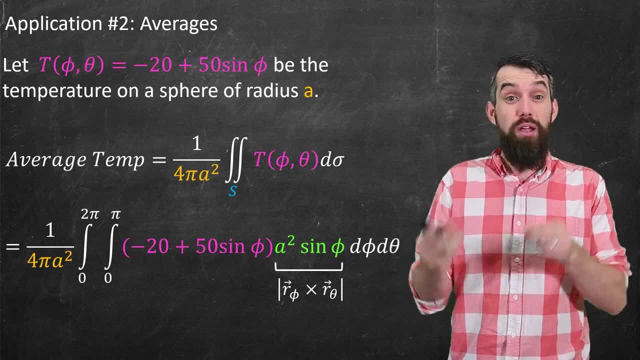 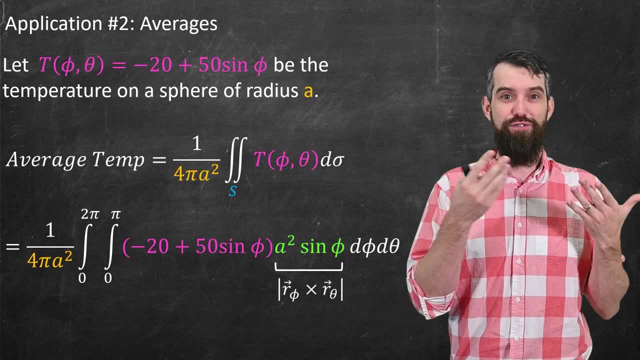 And we computed that before, As in a previous video, we computed the surface area of a sphere. We had parametrically described it in exactly the same way And we'd come up with this formula that we need to do when talking about surface area. 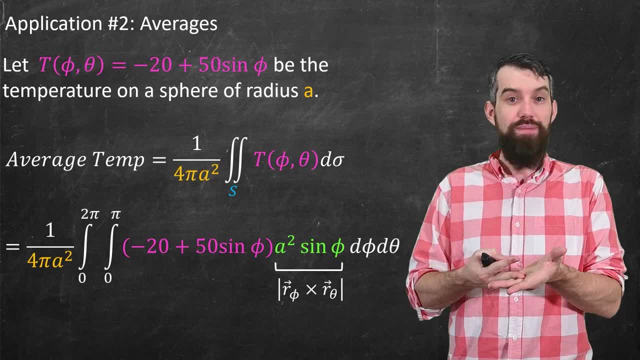 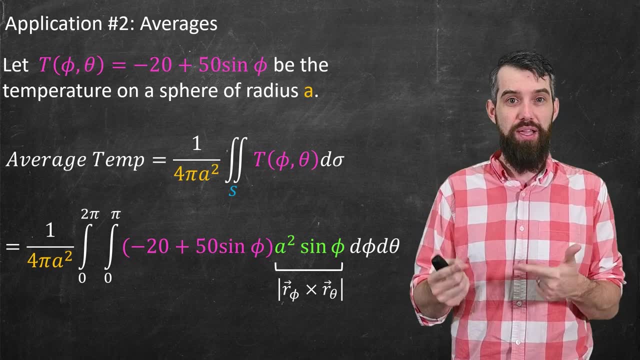 Parametrically, it's the r phi cross r theta. That exact thing comes up in surface integrals as well, And so, since I've already computed it, I'll just assert it for you. It was a squared sine phi. Now this is just a double integral.